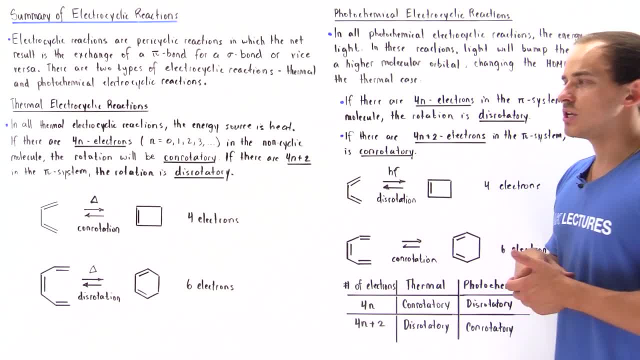 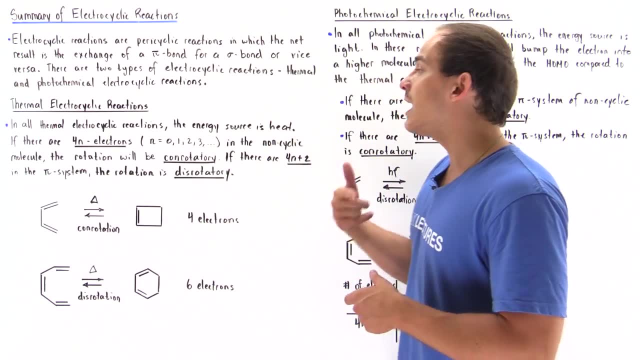 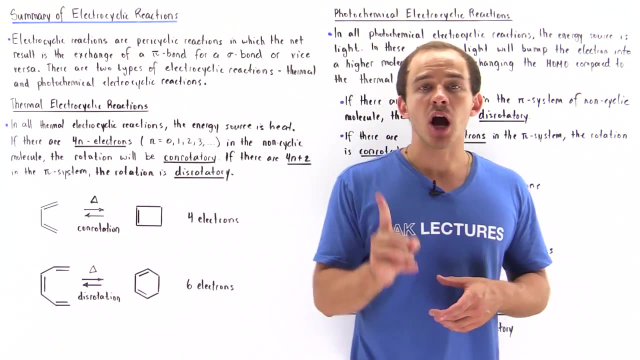 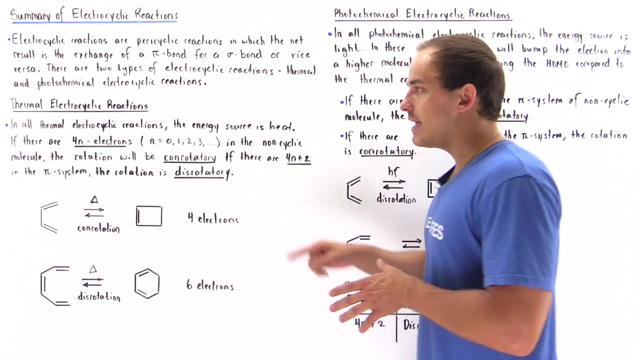 heat. Now, in some thermal electrocyclic reactions the type of rotation is this rotatory, In others it's conrotatory. So basically, what determines the type of rotation is the number of electrons within our non-cyclic molecule. So basically, if there are 4n number of pi electrons, where n 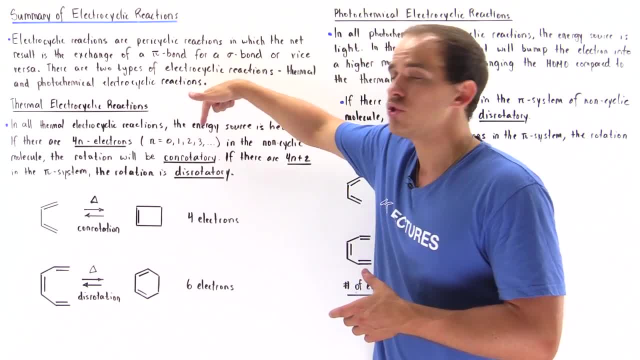 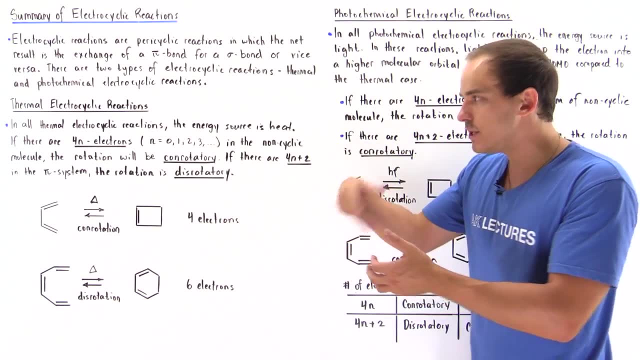 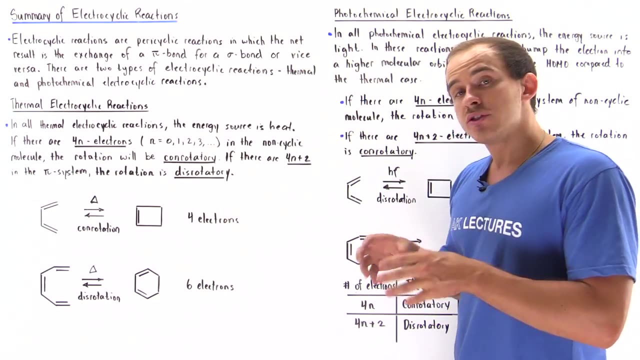 is basically a number that can be 0,, 1,, 2,, 3,, 4, and so forth. so if we have 0,, 4,, 8,, 12,, 16,, 20,, 24, and so forth number of electrons within our non-cyclic molecule, in that case the rotation- 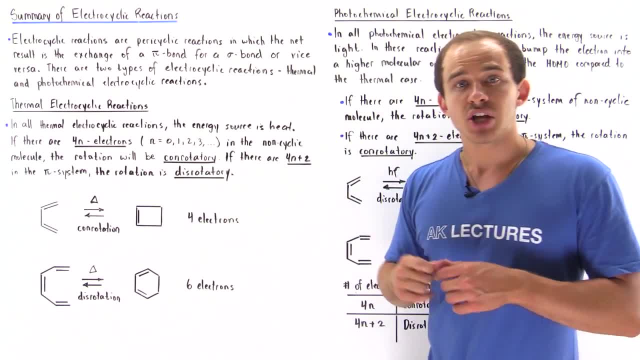 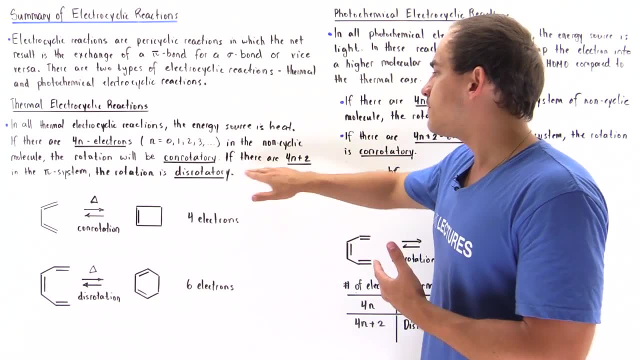 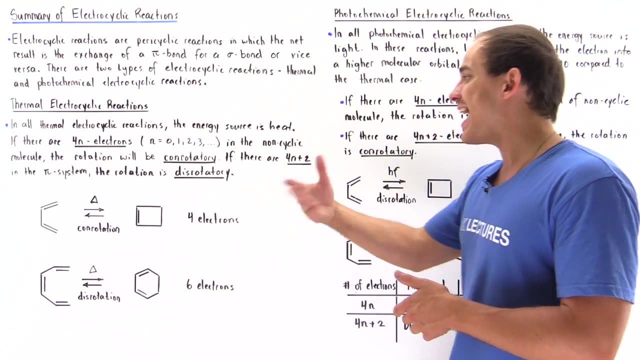 will be conrotatory, non-rotatory. So that means the two orbitals rotate either clockwise or counterclockwise. However, if there are four and plus two number of electrons, so 2,, 6,, 10,, 14,, 18,, 22, and so forth- 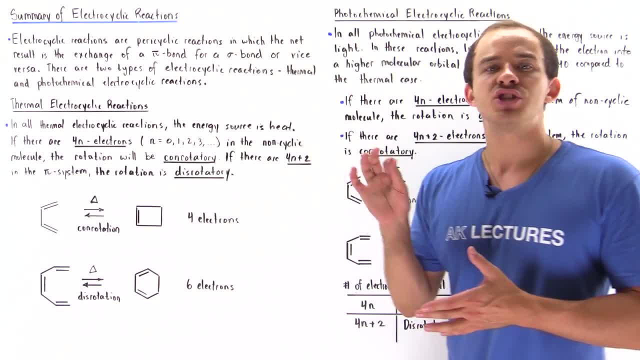 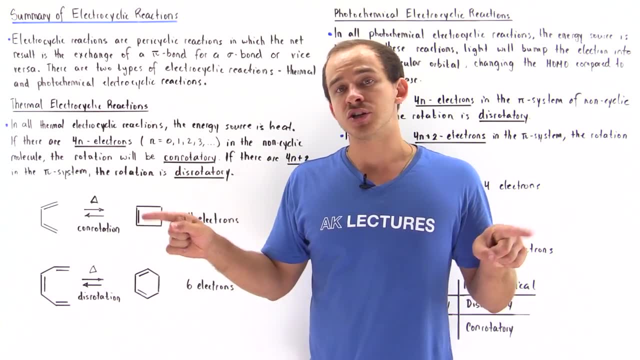 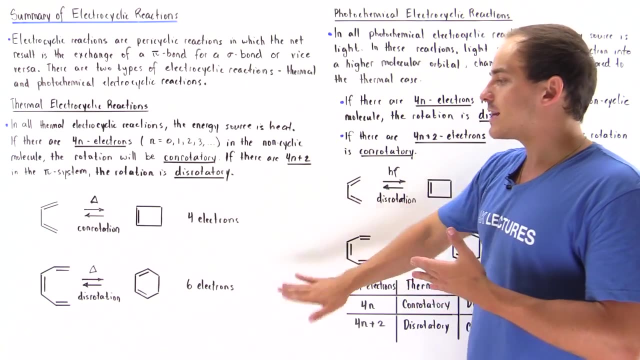 number of pi electrons, then the rotation is disrotatory. So that means the two orbitals basically rotate in the opposite direction. If one rotates clockwise, the other one will rotate counterclockwise. So let's take a look at the following two examples that we already discussed. 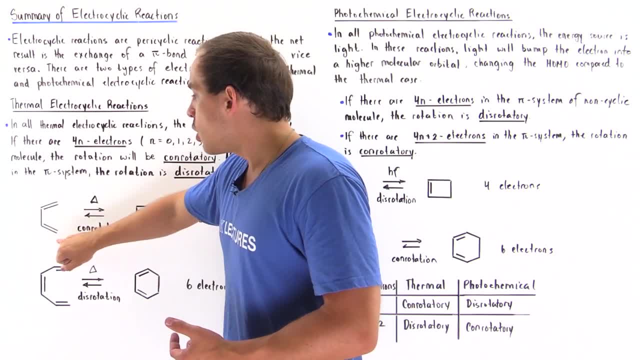 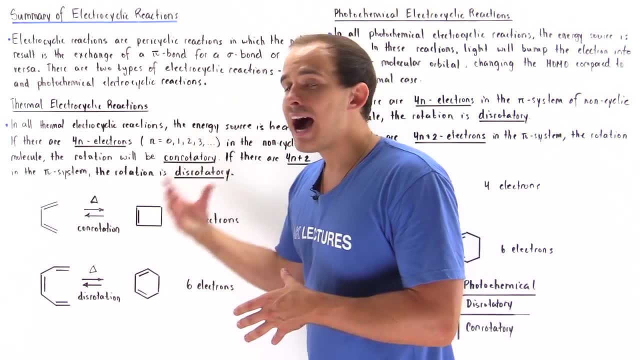 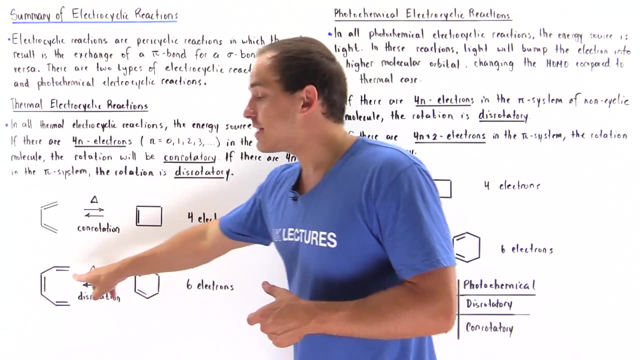 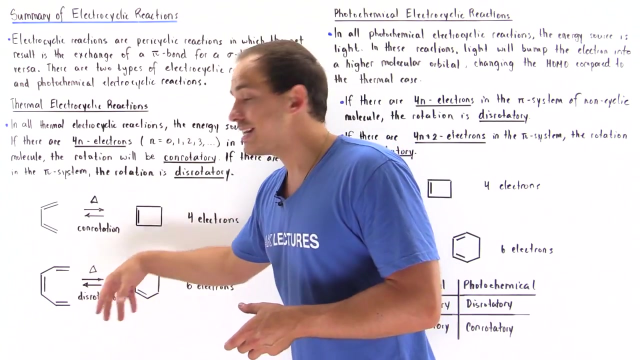 So we saw that if we take the following 1, 3 butadiene molecule and we reacted in the presence of heat, a conrotation will take place to produce this molecule. Now, if we take this molecule- 1, 3, 5, 1, 3, 5-hexatriene- and we mix it in the presence of heat, 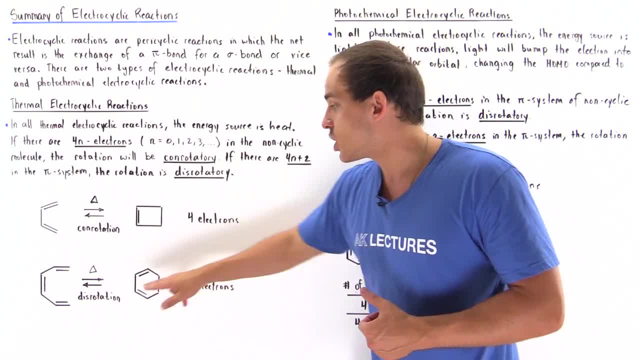 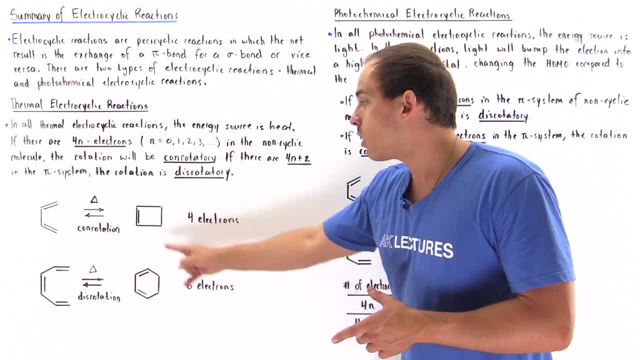 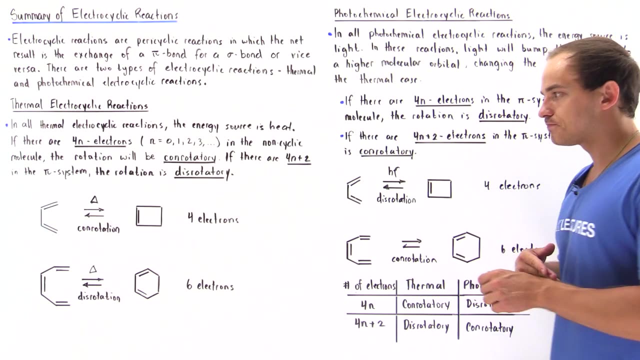 then we produce this molecule, in which we have a disrotation taking place to actually produce it. So if we have four electrons, that's a conrotation, If we have six electrons, that's a disrotation. Now what if we take this molecule and we react in the presence of heat and we react in the presence of heat? 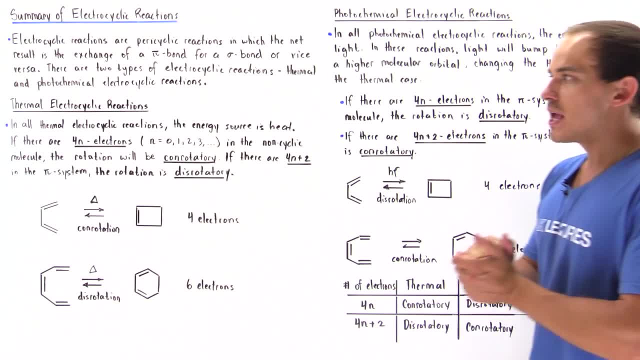 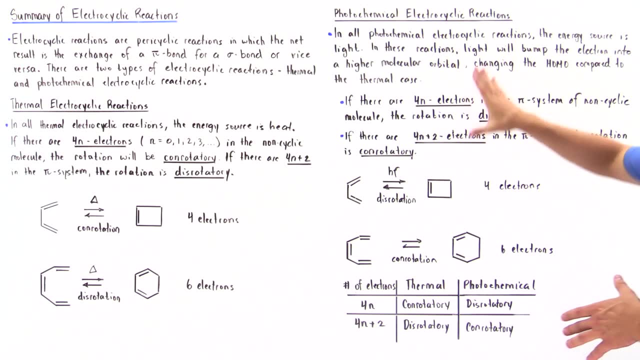 then the worl един happens. We have the Madam Hirst BH feature shocked, and this does not work over the. So the main difference between this and this reaction is: here we have heat as the energy source, but here- all photochemical, electrocyclic reactions, the energy source is light. 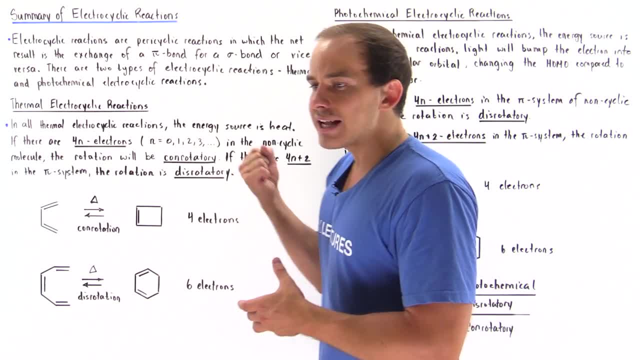 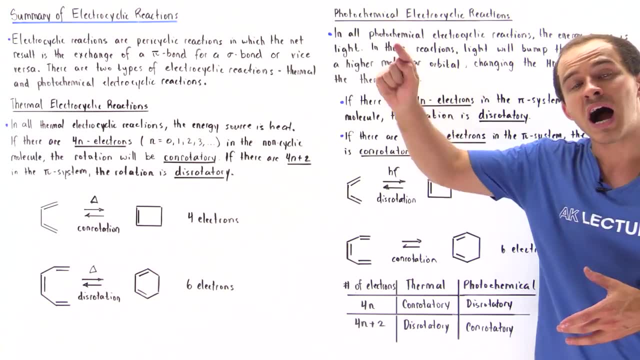 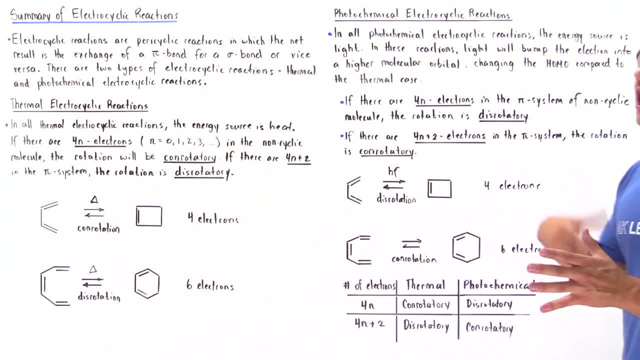 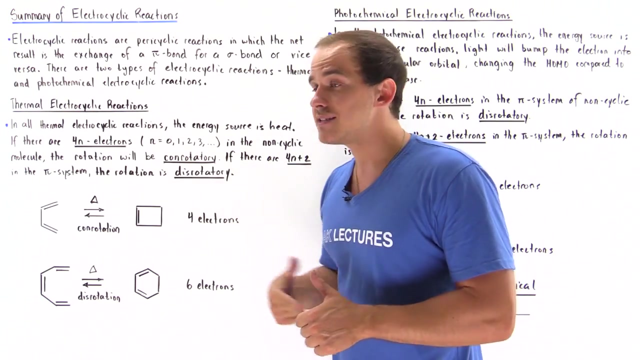 So in these reactions we basically shine light onto our molecular orbital and the electron jumps, it transitions to a higher molecular orbital. So the HOMO, the highest occupied molecular orbital in the photochemical case, is different than our HOMO, the highest occupied molecular orbital of the thermal case. 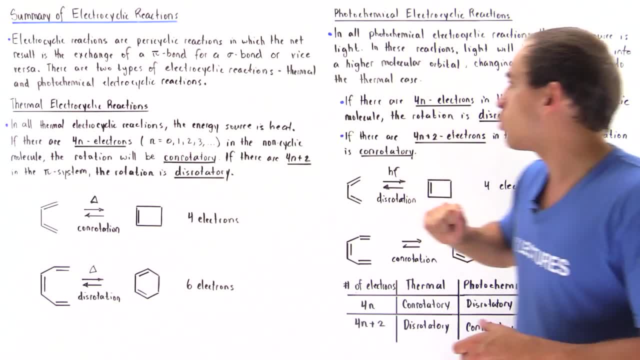 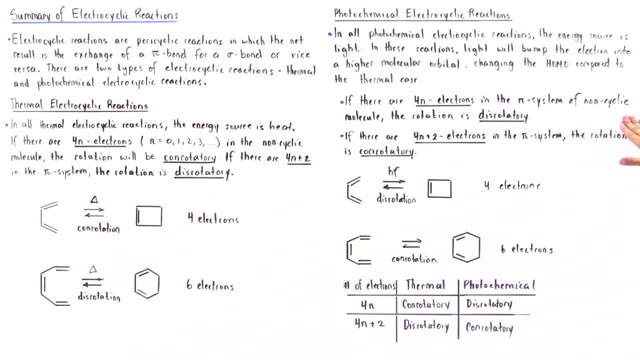 And that's exactly why these concepts are switched. So in this case, if there are 4n electrons in the pi system of the non-cyclic molecule, the rotation is not conrotatory, but it's disrotatory. And if there are 4n plus 2 electrons in the pi system, the rotation is conrotatory. 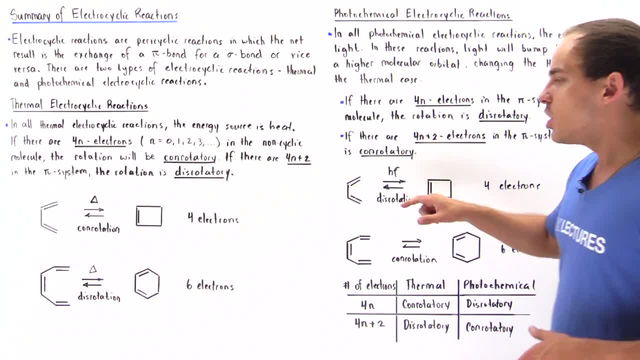 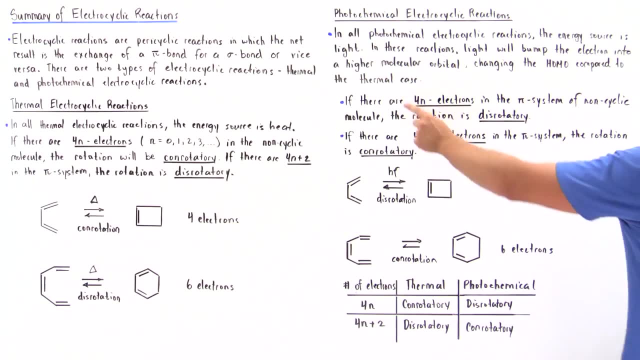 So basically, if we look at these same two examples, we basically switch these rotations, In this case because we have 4n. If we have 4 electrons, which correspond to n equals 1, our rotation is disrotatory. 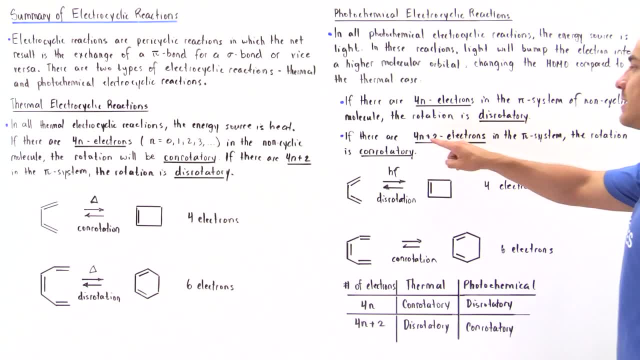 However, if we have 6 electrons, which correspond to 4n plus 2, where n is equal to 1, then it's a conrotation And this table here basically summarizes our results. So, if the number of electrons is 4n, for thermal reactions when we have heat as the energy, 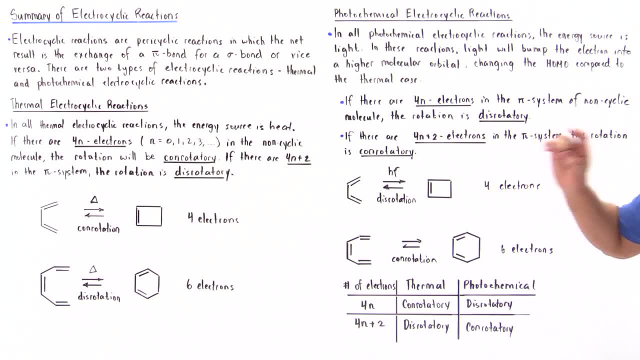 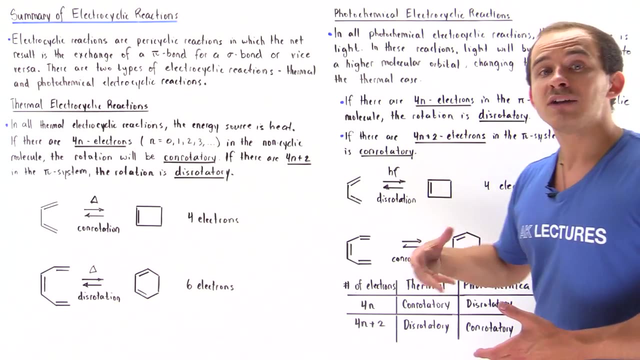 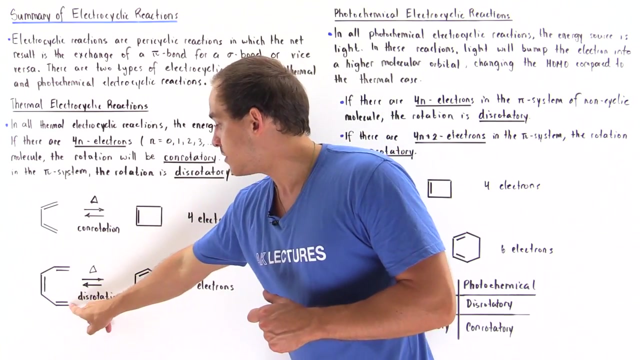 source. we have conrotation. for photochemical reactions, we have disrotation. Now for the 4n plus 2 case for thermal, we have disrotatory. for photochemical we have conrotatory. And once again, a conrotation is a rotation in which our two orbitals- this orbital and this orbital, and this orbital and this orbital.